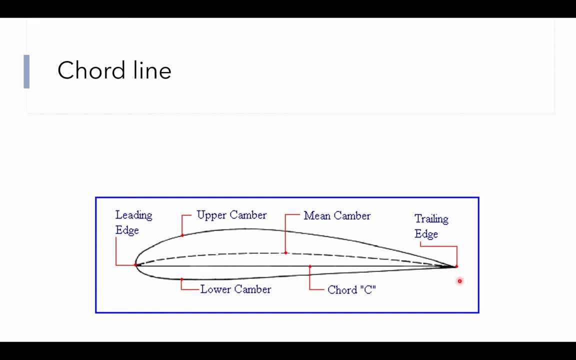 With those definitions in mind, we can talk about the chord line. The chord line is simply an imaginary line between the leading edge and the trailing edge of the wing. As long as you know where the leading and trailing edges are, you just need to play. connect the dots to find the chord line. The next term is camber. 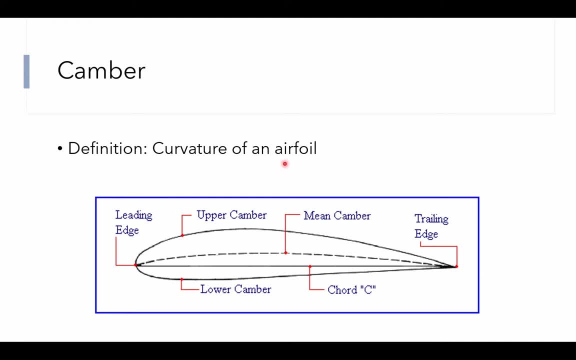 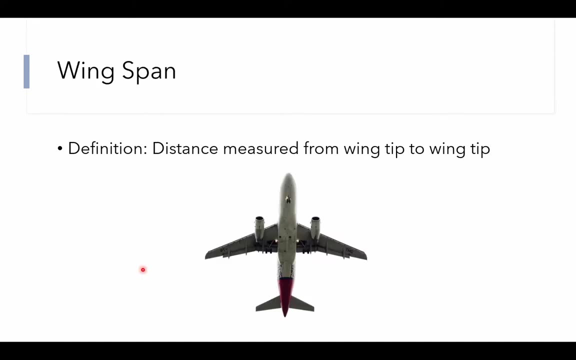 The camber is the curvature of an airfoil. In this diagram you can see that there are three cambers. The upper and lower cambers are just the upper curvature and the lower curvature respectively, And when you get an average, that is the mean camber. The fourth term is the wingspan. Wingspan is the distance. 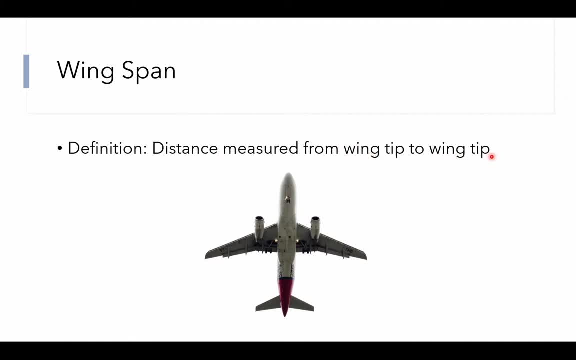 measured from wingtip to wingtip. This is another easy term. Again, just play, connect the dots with the two tips of the wing and you will get the wingspan. Next up is the wing area. The way to calculate the wing area is to calculate the wing area. The way to calculate the wing area is to: 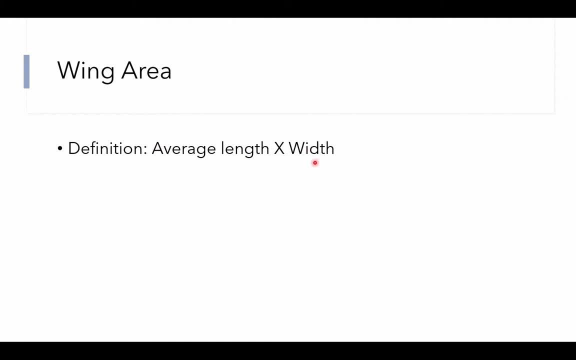 calculate the wing area is just by multiplying the average length by the average width. A good way to remember this is that it is the same as calculating the area of a rectangle. The next term is planform. Planform is the shape of the wing viewed from above. These are a couple of examples of wing. 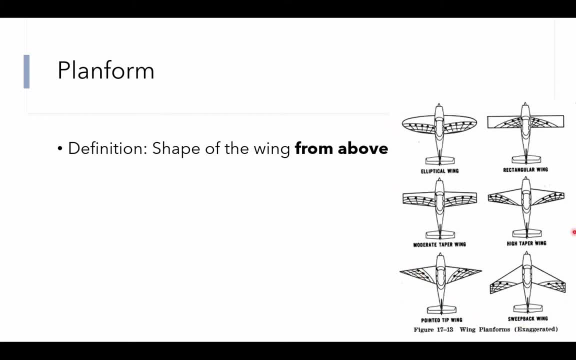 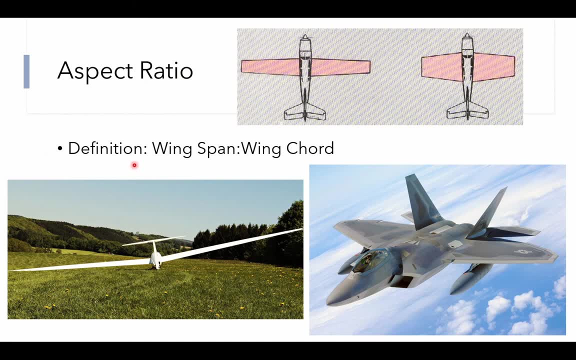 planforms. Up next is aspect ratio. The aspect ratio is the ratio of wing span to wing cord. Gliders typically have a higher aspect ratio because of their ability to reduce induced drag, while aircraft such as fighter jets have a low aspect ratio for their high maneuvering ability. The next term is the angle of 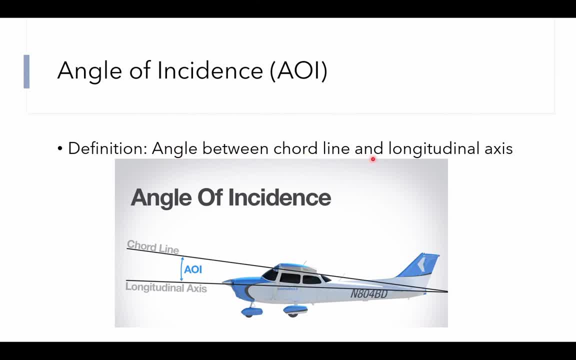 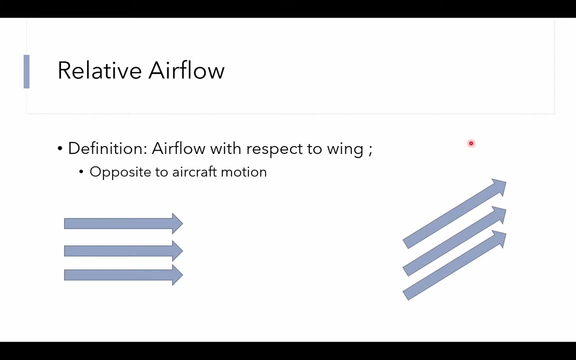 incidence. This is the angle between the cord line and the longitudinal axis. This is important as it defines your optimal takeoff speed. Do note that on most aircraft this angle is locked in place, so you really can't change it. Before we talk about the last term in this video, let's talk about relative airflow. 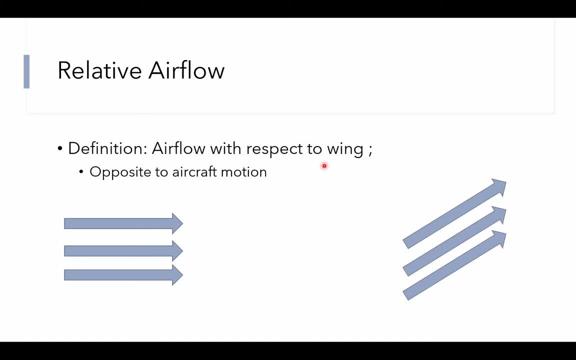 This is the airflow with respect to the wings. You can think of this as the airflow opposing to the aircraft's motion. When thinking about relative airflow, be sure to first ask yourself this: What is the aircraft's current motion In situations like stalls? although 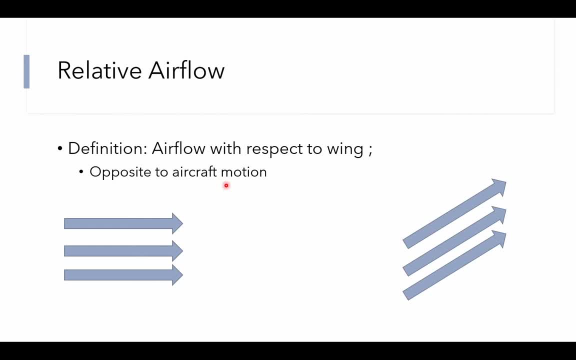 the aircraft's nose is up, the aircraft is actually dropping downwards, meaning that the relative airflow is not a horizontal line and instead in more of a 45 degree angle. This is very important, as it is crucial to understanding the last term, which is the. 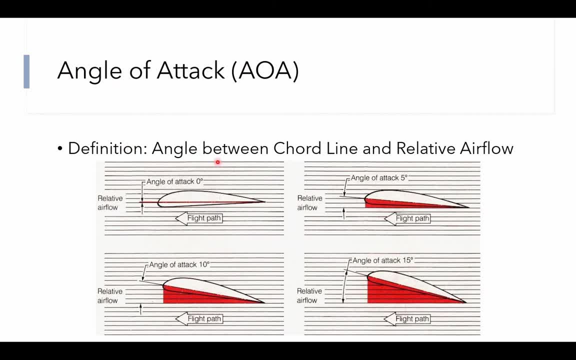 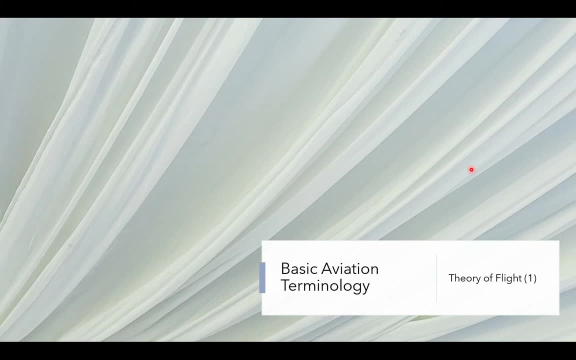 angle of attack. The angle of attack is the angle between the cord line and the relative airflow. This is a very important idea in aviation, as this determines a lot of what you can and cannot do. And that concludes this video. If you found it helpful, please consider liking this video. 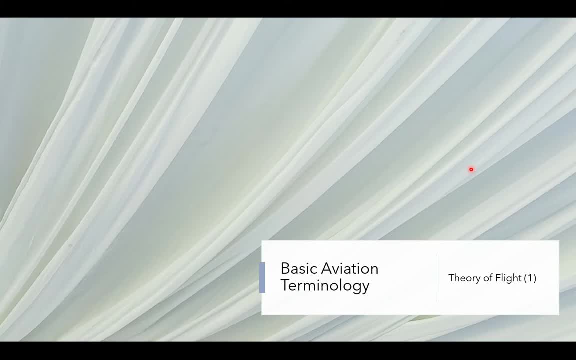 and subscribing to my channel. Feel free to also comment down below if you have any questions for me. I look forward to seeing you in the next video. 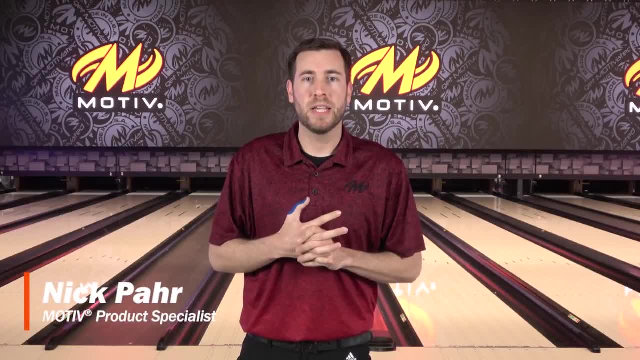 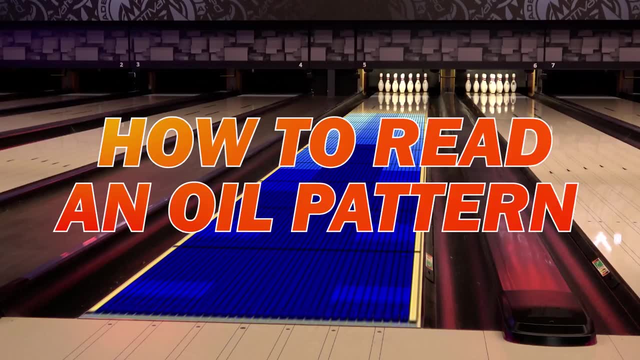 Hey everyone, Nick Parr here with you again in Grand Rapids, Michigan, at Spectrum Lanes, and today I'm going to be going over some tips for you on how to read the pattern without knowing the pattern beforehand. Typically, what I like to do is take my first three shots going over 5,, 10, and 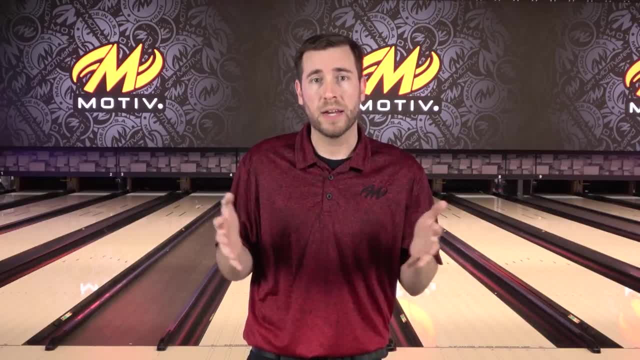 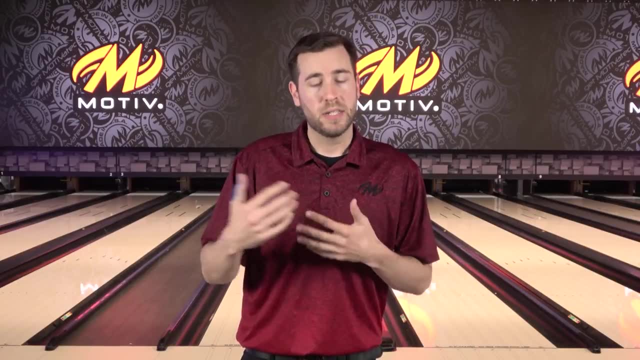 15 at the arrows. That just gives me an idea of what the pattern is doing and where I need to be, not only in the front but hopefully down lane as well. I'm kind of watching that as the ball is going down the lane, seeing where the ball is. 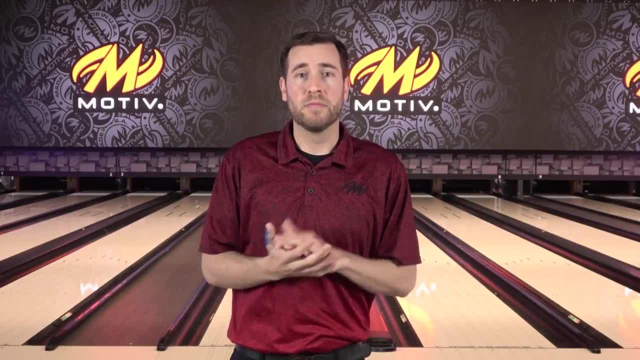 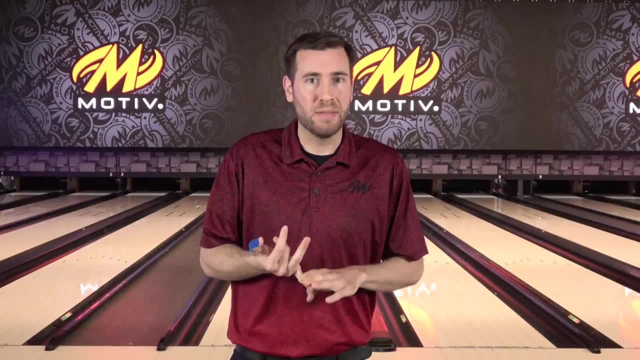 exiting the pattern, how it's exiting and all that. And the last thing I'm gonna be really aware of is actually watching the pins, how they fall and you know, in practice especially, what am I leaving. If I'm leaving a 10 pin, well is.